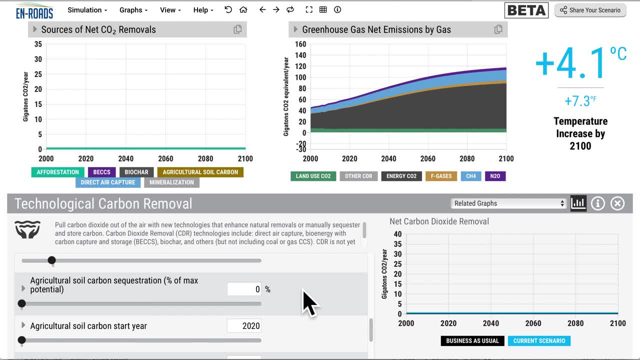 So what we're going to get if we move that to 100% will be a maximum of 5.5 gigatons a year, with some loss every year as some land that's in the best practices with low-till agriculture, leaves that designation. 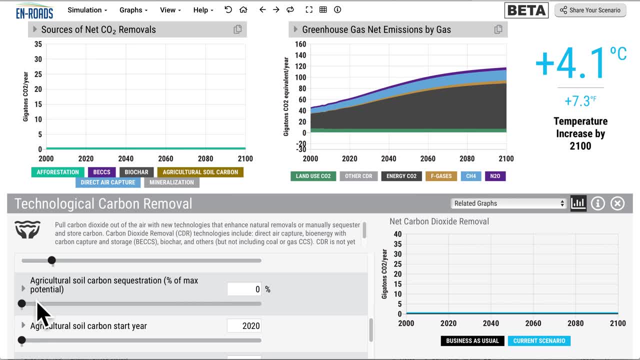 And you lose some of the carbon that had been stored. So here I am, I'm going to increase it up and we're going to watch up here to 100%. I'll run it again and you can see as it turns on and off this level and by 2040, we get up to about 5.5 gigatons per year of removals. 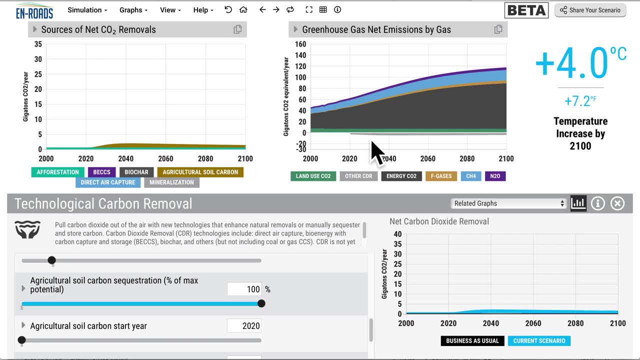 Where that shows up in the model is here with that see, that area below zero, That silver area, are the removals which go up to about 5, again gigatons of CO2 per year, pulling that much out of the atmosphere. 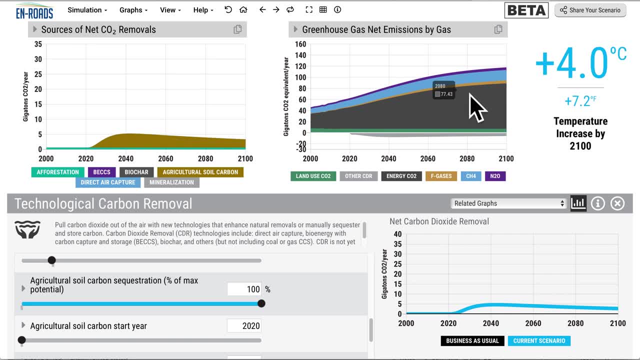 So what you have is everything above the zero line going in from land-use, CO2, this black area of energy, CO2, F-gases, methane, N2O coming out. Those are the removals: 5 gigatons a year and then declining over time. 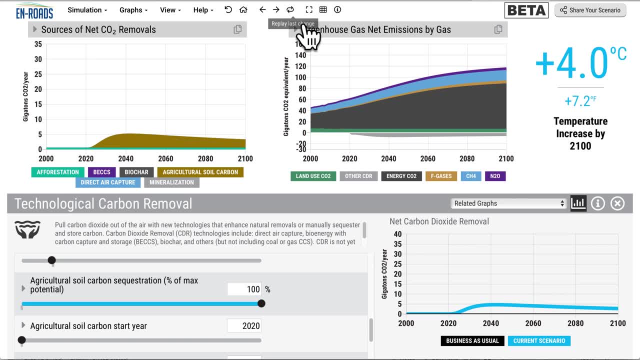 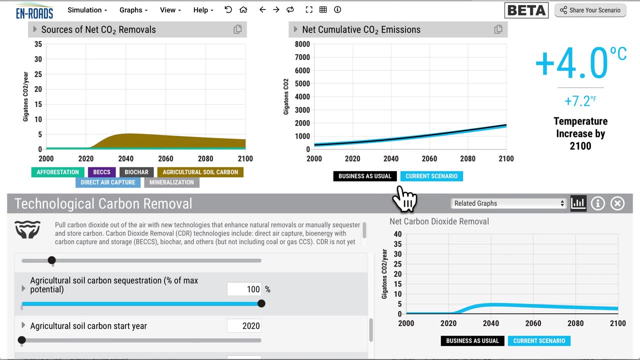 The result is about 0.1 degree, reducing temperature From 4.1 to 4.0,. we could also explore cumulative CO2 removed would be another way to look at it. So if we were to go here to CO2 emissions- net CO2 emissions, we could see what is the difference in cumulative net CO2 emissions for making that change. 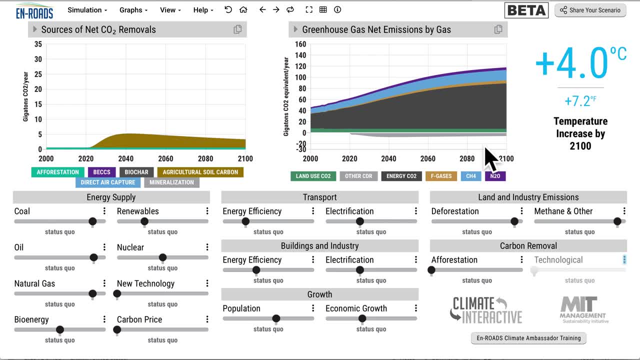 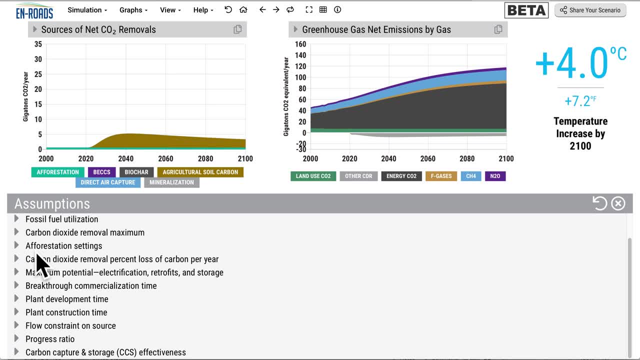 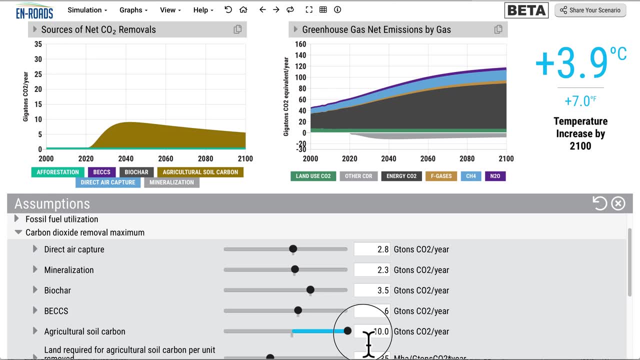 The loops on this assumption were higher if it was the high end of the Royal Society When we go down here to carbon dioxide removal maximum, and it was pushed up to 10.. You see the difference there between 5 and 10. It brings temperature down to 3.9.. 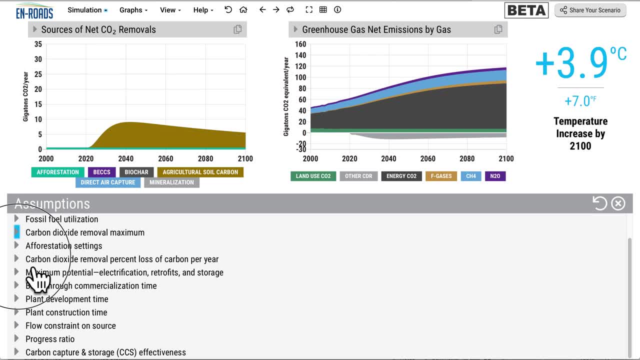 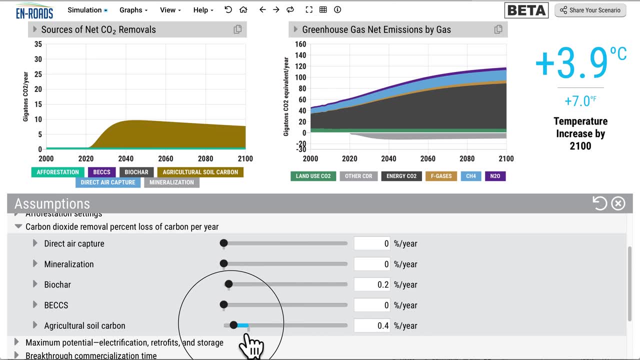 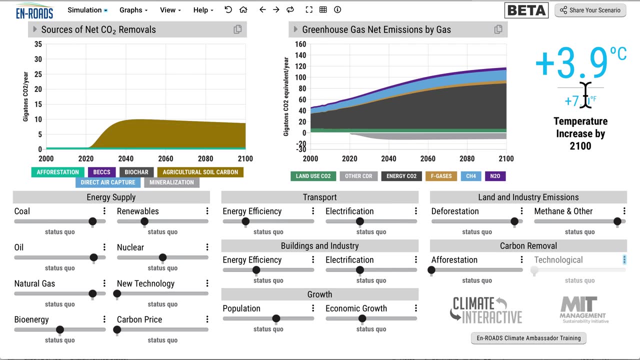 There are other uncertainties, such as the loss. What if the egg cell carbon loss isn't 1% a year, but a little bit less? You notice the different shape that you get. point three, and so there we are at bringing a change of 0.2. 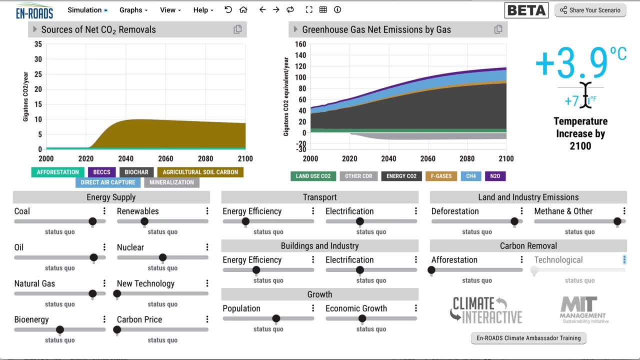 that is, uh, perhaps 10 of the way between 4.1 and getting to two degrees. you can debate all you like whether that's significant or not, but when you see what it takes to address climate change, there's no silver bullet. there's no one thing that's going to solve. 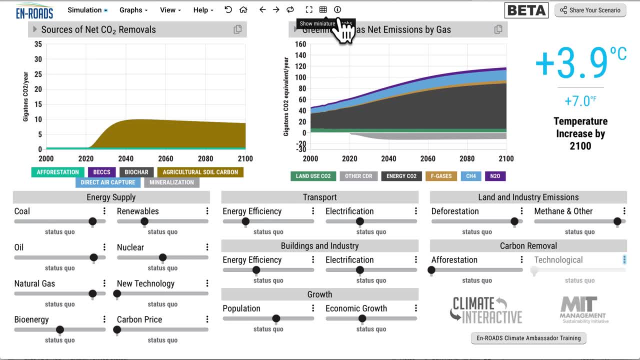 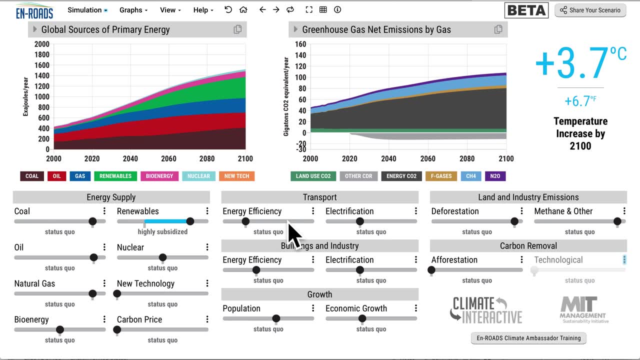 this problem, even when you supplement that with a variety of other actions such as incurring gene renewables, which helps another 0.2, and energy efficiency, transport is another 0.2, and buildings and industry, well, that's another 0.3. electrification gets us another. 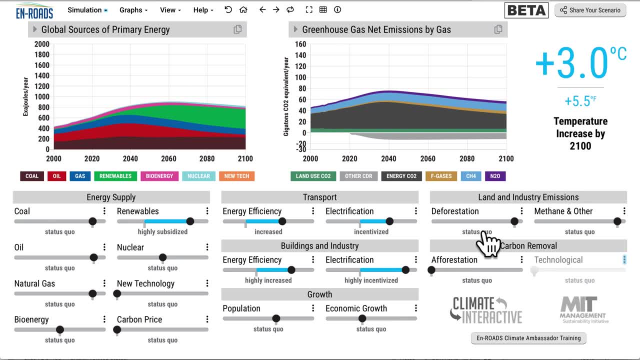 0.1 electrification here, another 0.1 or so deforestation, another 0.1 methane and other a little bigger, depending on how much you get of it. growing trees, we're at 2.4. setting a carbon price and keeping coal in the ground, you can see that it really takes many. 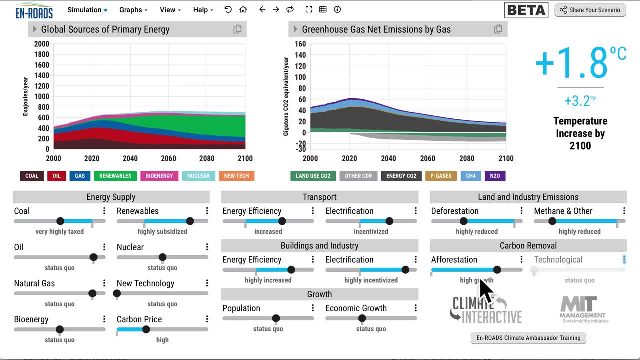 actions, many of which bring 0.1 or 0.2 reductions in temperature by 2100. put them all together and they could be part of a scenario that limits warming to well below two degrees. there's a lot more to say about the difference between keeping coal, oil and gas in the ground.